And fractionate it accordingly. But if this were much colder, you would remove a much larger fraction, maybe three quarters of the water vapor. That would fractionate more strongly and you'd get lighter isotopes falling on the ice sheet. So temperature, remember controls, how much water vapor? you have in the atmosphere. So the more cooling you get, the more water vapor has to be removed. The more water vapor you remove, the more fractionation there's been in the isotope ratio. OK. So it's remarkable that these two local records of fractionation and temperature are so similar, They provide an accurate time record of the ice ages. One more thing that's even more astounding: you can take those same ice cores and find tiny bubbles in them As the snow fell. and more snow fell on top, and you finally. compacted it into ice. there are little bubbles that trap samples of the ancient atmosphere. You can stick a probe into those ice bubbles and do a carbon dioxide concentration analysis to find out what the carbon dioxide concentration was in those ancient atmospheres. So here I've plotted up from the Vostok core alone a. record that goes the time axis is switched here. This is today and this is going back in time. This goes back a bit further. I've shown you data back to 400,000 years ago. Here's the isotope record converted to a temperature. isotope record, converted to an equivalent temperature and then in the top panel is the carbon dioxide concentration taken from the same location along the ice core. Here's the modern day. At the top of the ice core you had about 280 parts per. million by volume, which is about the value we think is the pre-industrial carbon dioxide value for the Earth's atmosphere. Then, back into the last ice age, the last glacial maximum is here. you had much lower carbon dioxide concentrations, even below 200 parts per thousand. 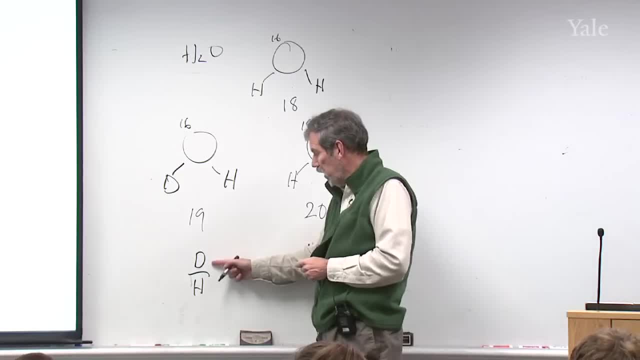 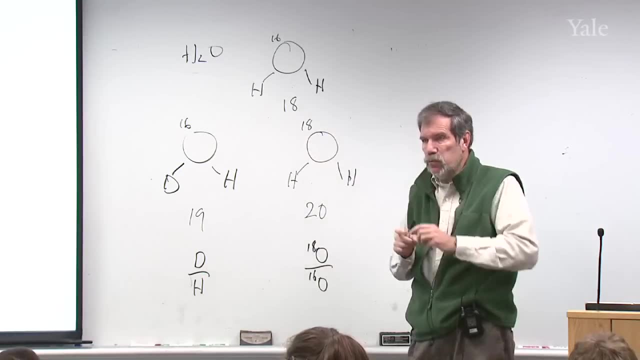 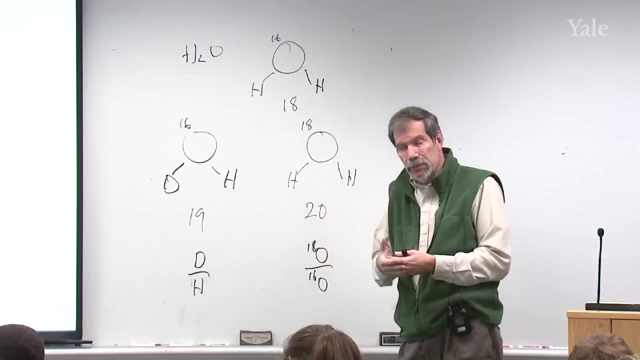 It stayed low. In other words, it mirrored the temperatures. quite remarkably, Carbon dioxide concentration and temperature are very similar to a very similar record, at least over this period we call the Pleistocene, where the ice age is coming and going and coming and going, which well we'll. 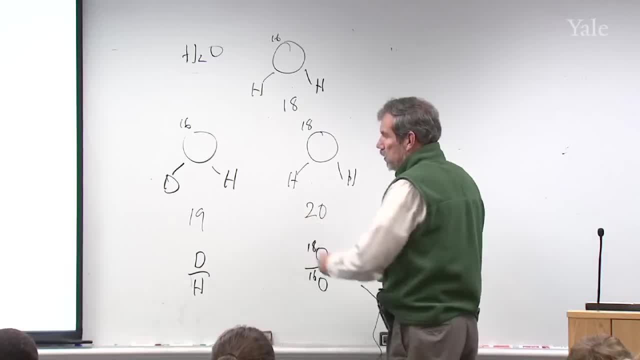 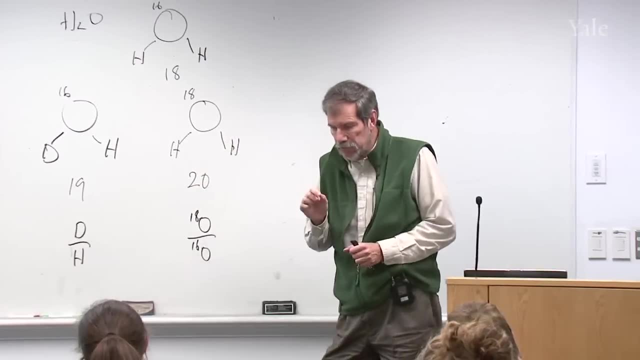 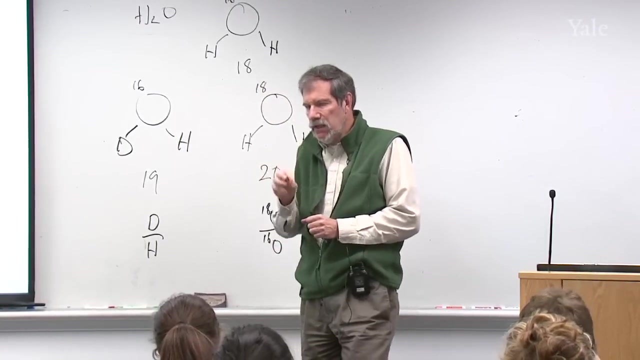 talk a lot about this coming up in the global warming, but at a very minimum. this reinforces our idea of the importance of CO2 in climate. When you had high CO2, you had warmer climates. When you had low CO2, you had colder climates, perfectly. 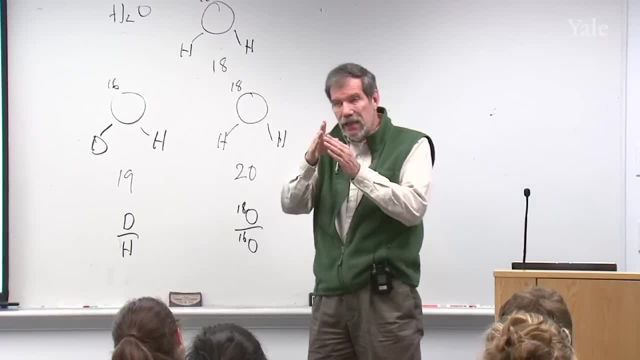 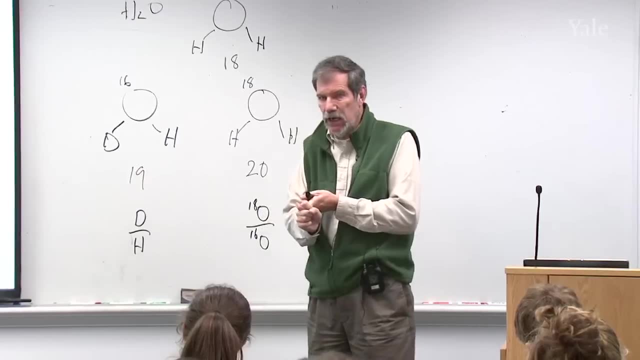 fitting with our idea of the greenhouse effect And CO2 being a greenhouse gas. Now there's also some argument, though, about cause and effect. which comes first, which leads and lags? We'll get into that a little bit next week. 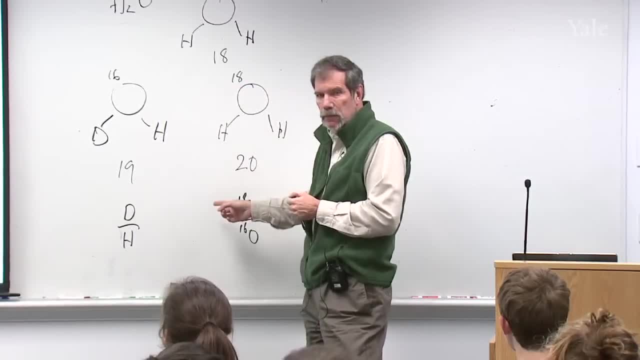 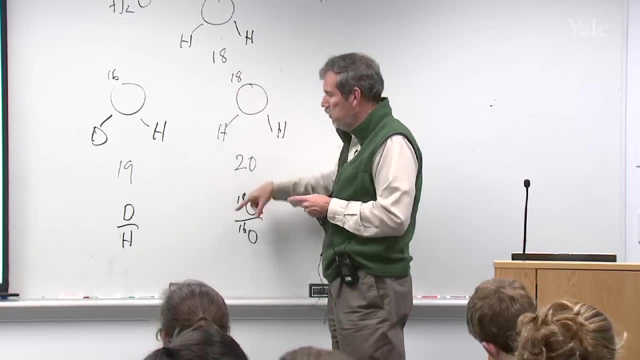 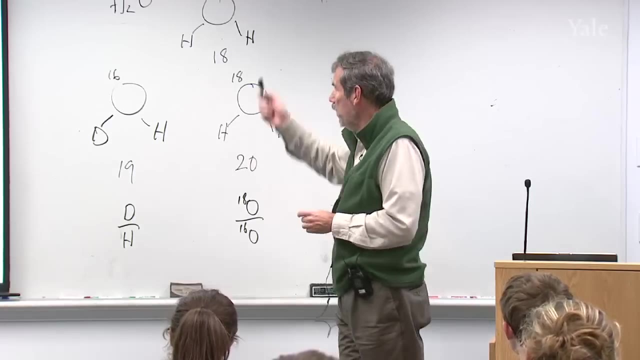 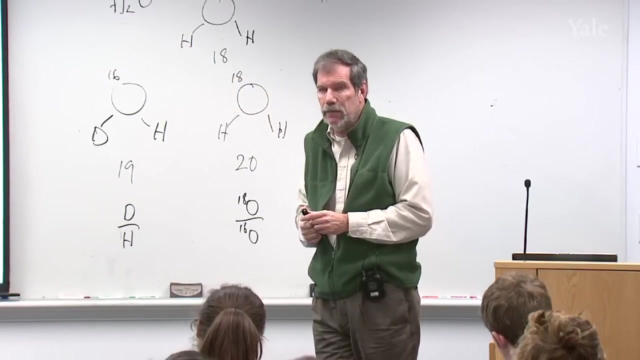 But for the time being I would take this at face value and just say that it reinforces the connection between CO2 and the atmosphere and global temperature. Now I want to talk about other kinds of sediments On land. you can walk around and see rocks like this. I'm 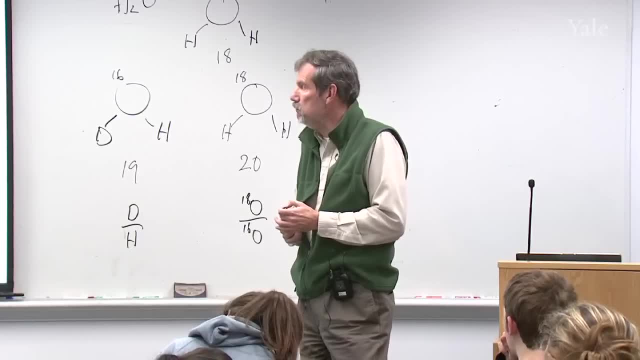 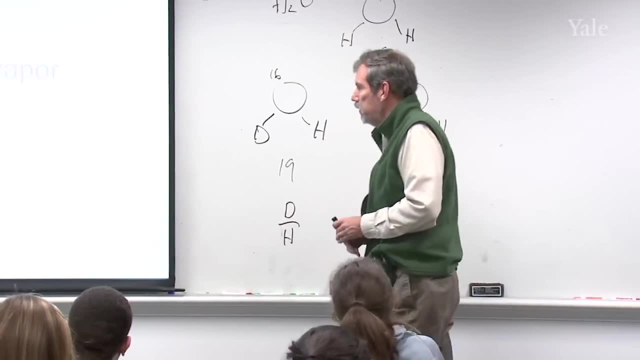 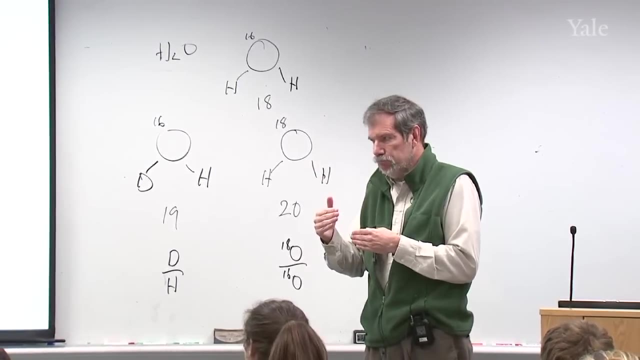 sure you have rocks that seem to have a layered structure. Most of the time when you see such rock patterns, you're looking at some kind of evidence of ancient climate change. One kind of climate allowed sediments in a lake to look like this. a change in climate changed it to that a change. 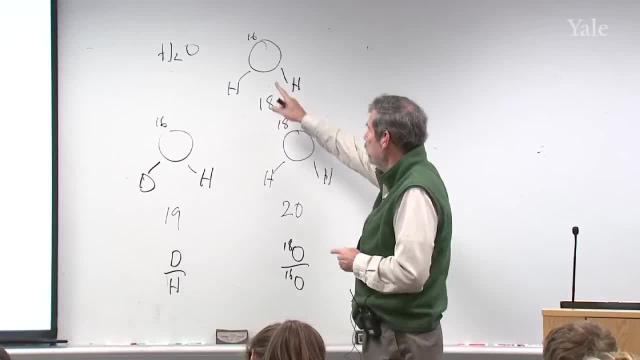 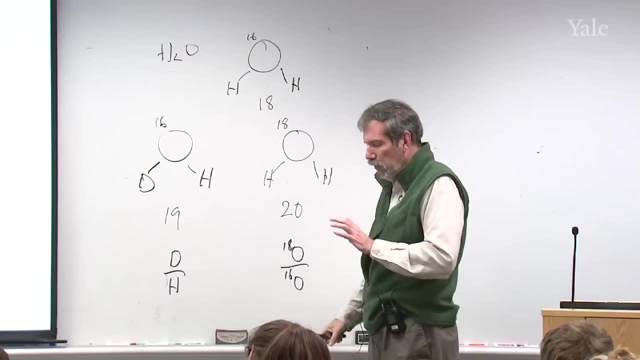 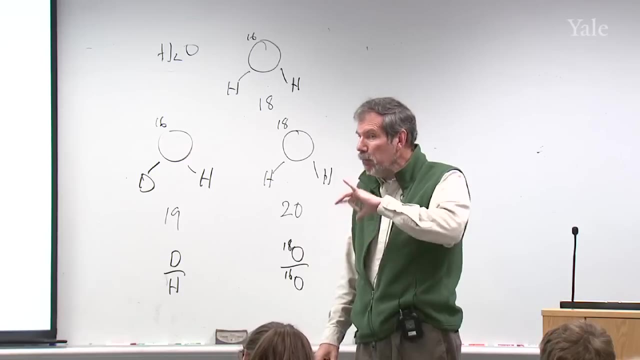 back, A rock gave sediments like this. This is easy to speculate about because you see lots of sedimentary layered rocks like that. It's not so easy to figure out what exactly this means in terms of climate, But it's a start to be able to see such stratification on land. 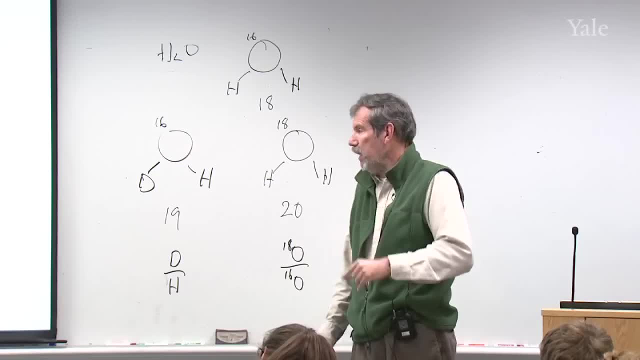 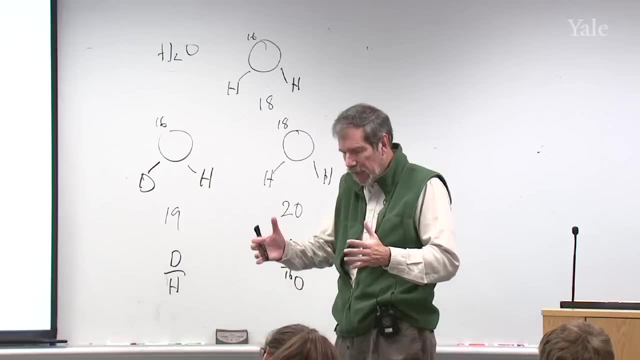 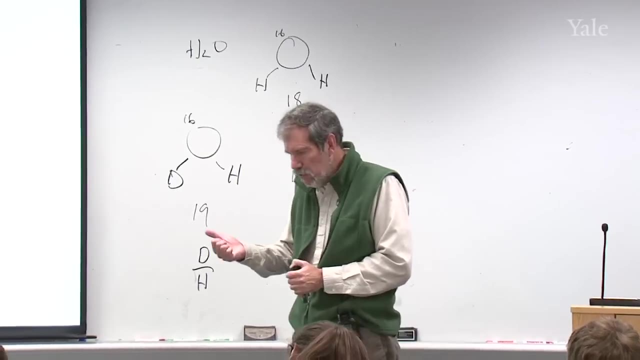 and just imagine in a vague way that, hmm, this may be evidence of changing climates in the ancient world. How many have been to Grand Canyon? Well, you have. You see something like this and lots of layered rocks, And what you should be thinking of when you see rocks. 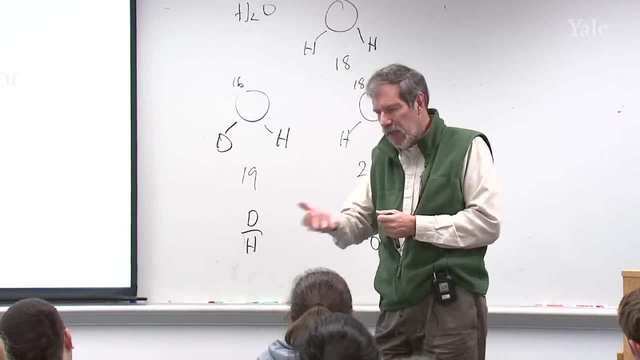 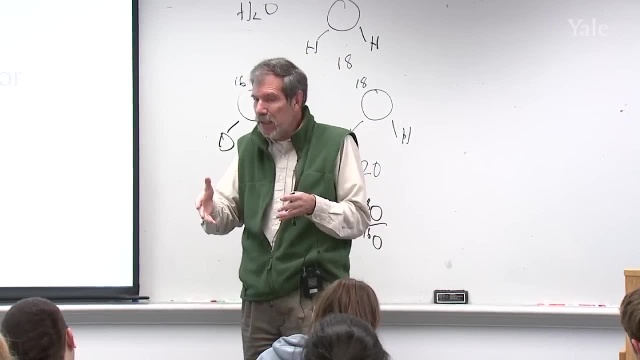 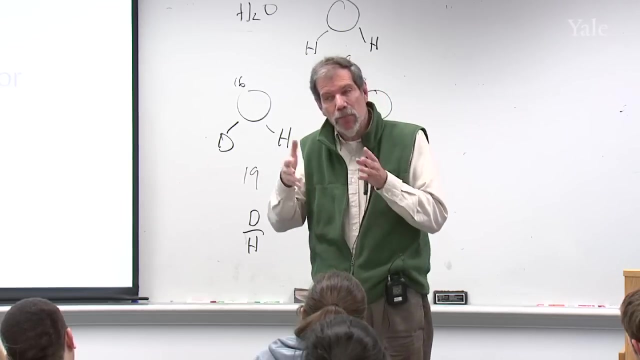 like this is ancient climate change. These changes probably are telling us something about changes in the ancient climate of the Earth, But again, they're rather difficult to sort out because we don't always know the environment in which those sediments were laid down. 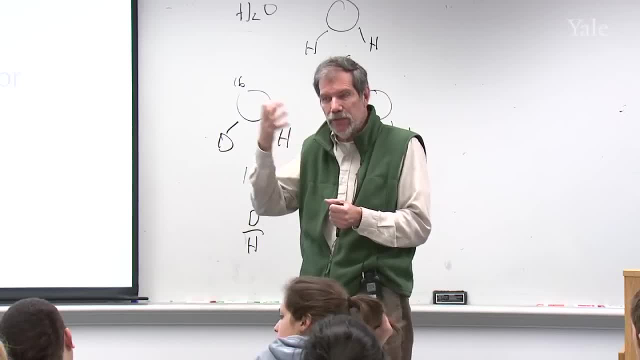 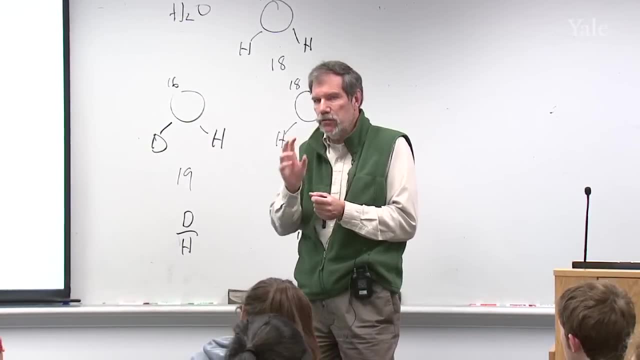 So we're going to do something similar to this, but in the ocean, where the ocean sediments have had a rather constant sedimentation rate And therefore we can do a little easier job of interpreting if we can get a sample of that. 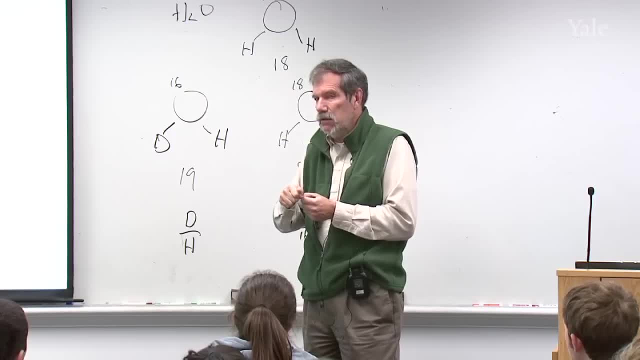 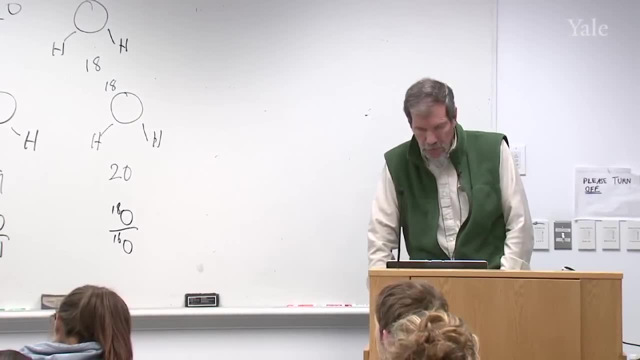